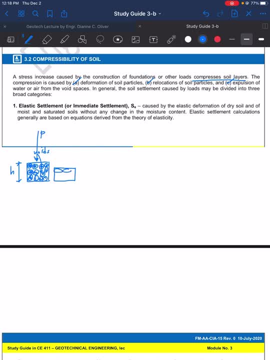 So, for example, it flattens out like this, like a pancake Flattens out. Thus, in this volume of soil particles there exists a change in height. So this change of height is our settlement or the compression of the soil layer. So this is due to deformation of the soil particles. Now the same. Now the second one is the relocation of soil particles. So why does relocation of soil particles cause compression? So again, let's have here a soil sample of a given volume. 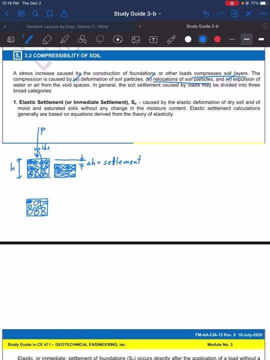 So these are the soil particles. So in this volume of soil, same with the first one, here quite a bit contains solid particles and voids here, voids which contains air, water, etc. okay, so in our second cause of compression since their relocation of soil particles. so upon introducing a force p 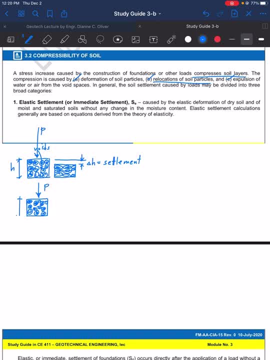 on top of the soil layer of height h there is a relocation of the soil particles. so in this volume, the soil part, because of the force the soil particles find, or some of the soil particles start to look for void spaces on its neighboring area and they start to fill it. thus, 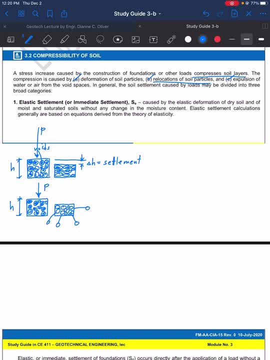 these soil particles are removed from the, from the soil sample. so there causes a delta h or the settlement, the change in height or the, then the existence of the compression. okay, so the soil particles are relocated, but if you notice, there still exist voids in this soil sample. so voids are still in there, but some of the particles have relocated. 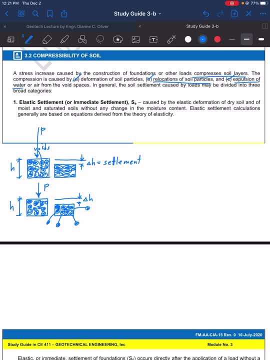 now the third one is expulsion of water or air from the void spaces. so let's take again example: a volume of a soil sample here of solid particles containing solid particles and voids. so we have here height h if we expose this solid, this soil sample, on a force p. 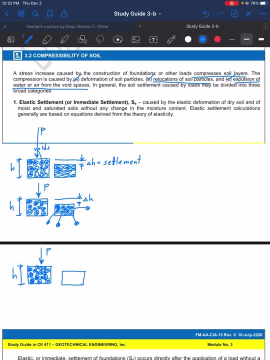 what happens here is the removal of the void spaces. it becomes denser because the content of solid particles are still there. so there is no expulsion of solid particles. the only ones that has been expelled are the, the uh, the voids, the uh water. what i mean is 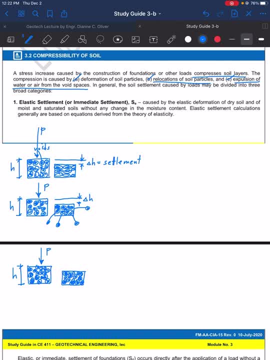 the only thing that has been expelled is the water or air from the void spaces, so this becomes denser and a delta h or settlement occurred or compression occurred. so these are the causes of compression. so in general, the soil settlement caused by loads may be divided into three broad categories. the first one: we have the elastic settlement, or the 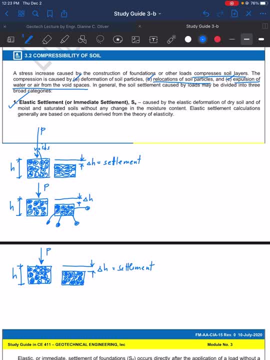 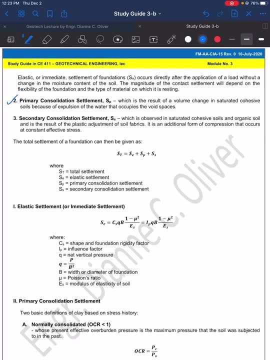 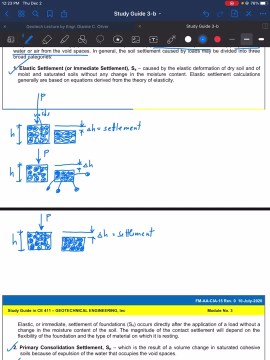 immediate settlement with the symbol s sub e. the second one: we have the primal consolidation settlement with the symbol s sub p, and we have the third one secondary consolidation settlement with the symbol s sub s. so let's differentiate these three. the first one: we have the elastic settlement or immediate settlement. so you can notice here elastic. 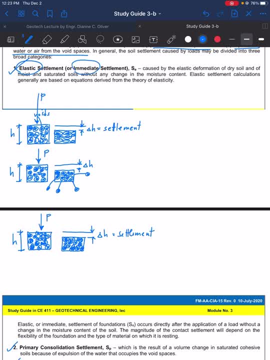 and immediate words. so what do we mean by elastic settlement or immediate settlement? it is caused by the elastic deformation of dry soil and of moist and saturated soils, without any change in the moisture content. elastic settlement calculations generally are based on equations derived from the theory of elasticity. 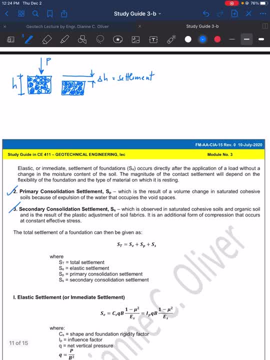 elastic or immediate settlement of foundations s of e occurs directly after the application of a load, without a change in the moisture content of the soil. the magnitude of the contact settlement will depend on the flexibility of the foundation and the type of material on which it is resting. 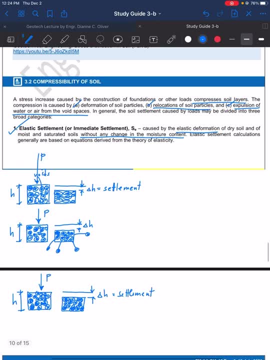 so why is it like that? well, let's go back to the definition of elastic deformation. what do we mean by elastic deformation? so when we say elasticity, it is the ability of a body to resist a distorting influence and to return to its original size and shape when that influence or force, force is removed. 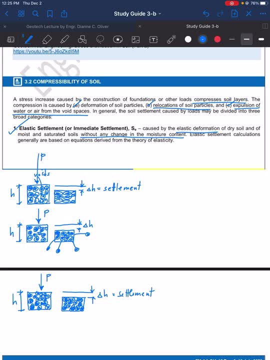 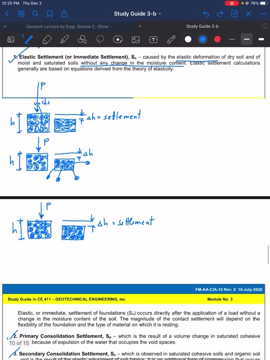 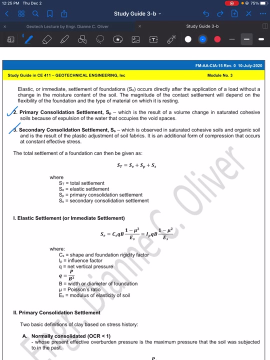 okay, so meaning it is a settlement, because it can go back to its original size, and it's also notable that this is the first settlement that we can observe in a soil layer because of the word immediate settlement. okay, so this is the settlement that is noticeable in a short period of time. for example, if you 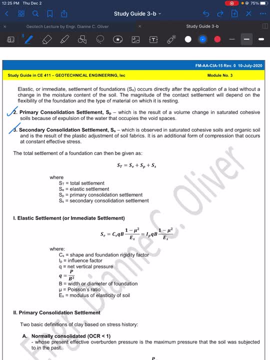 there's an area, your construction site, you load it up with piles of steel bars so that soil area experience, the first settlement, which is the elastic settlement experience is changed in age, which in some time, if you remove that load, for example that pile of steel bars, if you remove those loads, 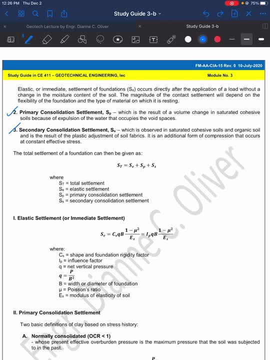 there's a possibility of the soil layer to return to its former shape or to return to its former height, and then that Delta H can become negligible. but still it is not worthy to compute for Delta H for for determining the settlement on that area. okay, so the first that we are going to solve is the 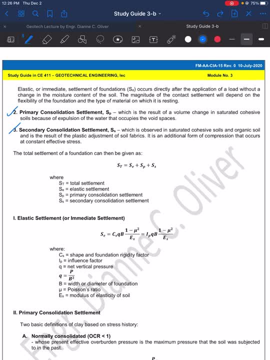 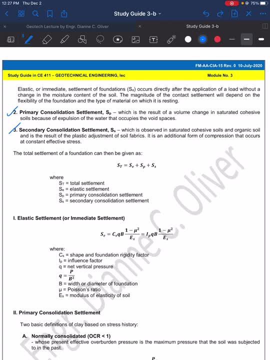 the void spaces. so here the voids, the void spaces has been reduced because of the expelling of the water and air. okay, so here in our primary consolidation settlement. this comes right after settlement, because if the loads are left there for a longer period of time, the voids can be removed. so the voids can be removed. number three: 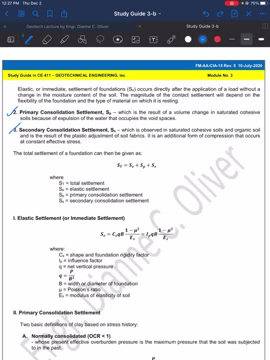 secondary consolidation settlement. symbol S: the S sub S, which is observed in secondary consolidation settlement. symbol S: the S sub S, which is observed in saturated cohesive soils and organic soil and is the result of the plastic. saturated cohesive soils and organic soil and is the result of the plastic. 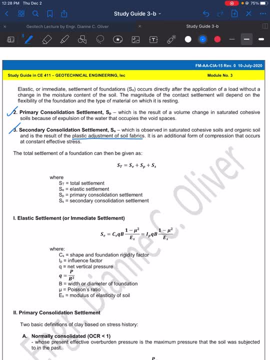 adjustment of soil fabrics. it is an additional form of compression that occurs at constant effective stress. now take note of the word plastic. that occurs at constant effective stress. now take note of the word plastic. adjustment. so what's the difference, again, between elastic and plastic? okay, adjustment. so what's the difference, again, between elastic and plastic? okay, so elastic is誠. 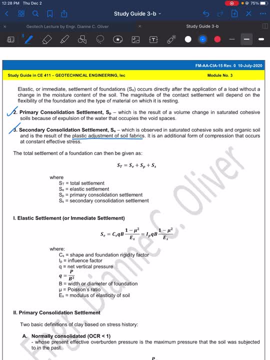 temporary. but when we say plastic, okay, the material will experience permanent deformation, okay. so in this settlement, this kind of settlement, the soil layer experiences a permanent deformation. so this happens when the uh, the load that is being experienced by the soil layer or by the soil, is happening over an extended period of time. so in the in this uh, 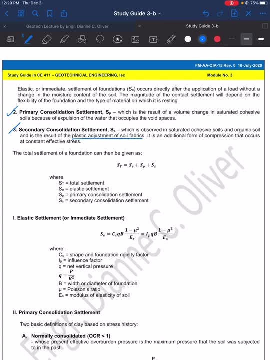 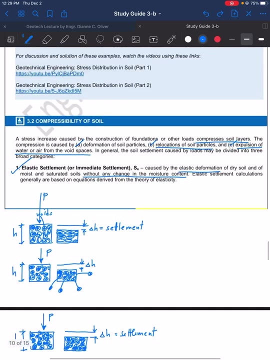 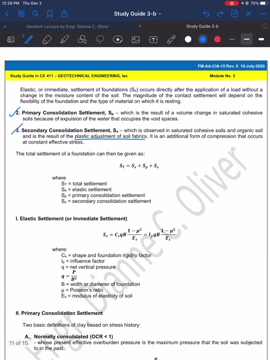 third category, we will incorporate the the parameter time to experience the plastic adjustment of soil fabrics. okay, so we have these three broad categories: the elastic settlement, the primary consolidation settlement and the secondary consolidation settlement. if you add them up, that is the total settlement. okay, let's go to the formulas for this. 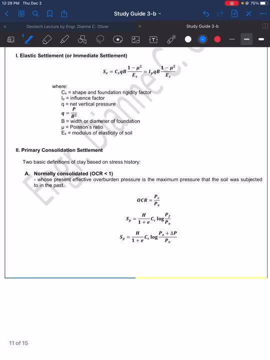 uh, three categories of settlement. the first one, the elastic settlement or the immediate settlement. so the formula for elastic or immediate settlement is: s sub e is equal to c s small q b times one minus mu, squared over uh. e sub s whole over e, and that is also equal to. 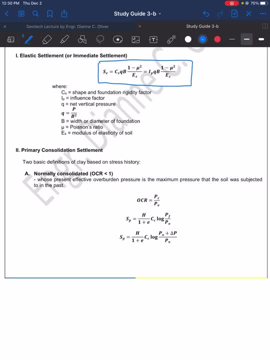 one minus uh mu squared. x e s. okay, uh, i don't hope i pronounce this correctly. okay, for the c sub s, that is our shape and foundation rigidity radiety factor. the哪裡 sub p is our influence factor. we have small q as the net vertical pressure and we have here: 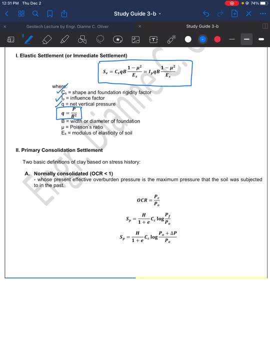 the formula q is equal to p over b squared, where p is the load and b is the width or diameter of foundation, and then this mu here is the poissons ratio, and then e sub s is the modulus of elasticity of soil. okay, the second one is the primary consolidation settlement. 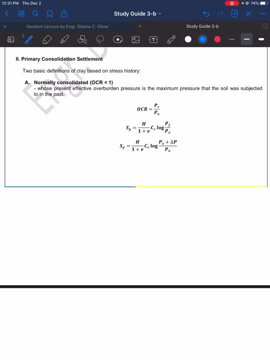 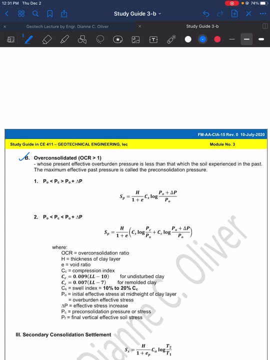 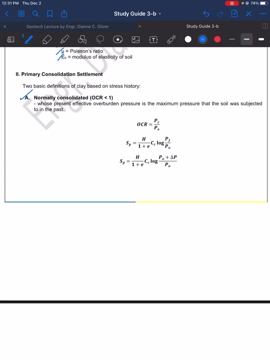 we have two basic definitions of play based on stress history. we have the normally consolidated in which ocr is less than one, and then we have the one here, the over consolidated, where ocr is greater than one. okay, so this first one. here we have the normally consolidated wherein ocr is less than one. so what is ocr? 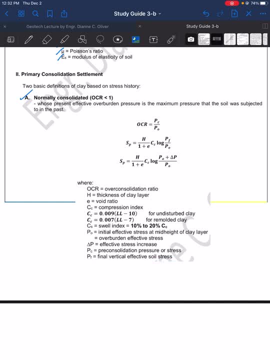 so ocr is the over consolidation ratio. then over consolidation ratio is equal to p sub c over p sub o. what is p sub c? p sub c is pre-consolidation pressure or stress. p sub o is the initial effective stress at mid height of clay layer. it is also called the overburden effective stress. 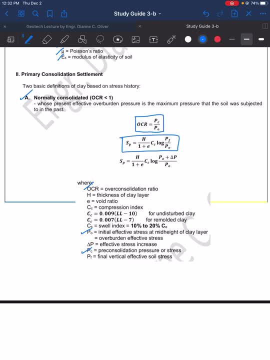 then we have the formula for the settlement, primary consolidation settlement: s sub b is equal to h over one, plus e, c sub c. log of p sub f over p sub o, where h is the thickness of clay layer, e is the void ratio, c sub c is the compression index and we have formula for: 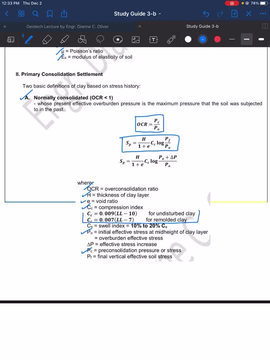 compression index. we have two. okay, so the first one. so the first one is c sub c is equal to 0.009 times liquid limit minus 10.. and this formula is for the undisturbed clay. the second one we have: c sub c is equal to 0.007 times liquid point. 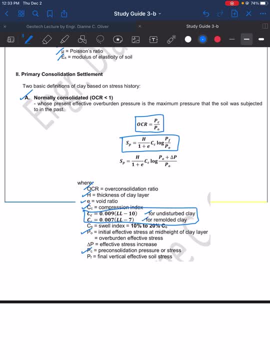 limit minus seven, and that is for remolded clay. okay, so that's the formula. and then we also have here c sub s, the swell index. that is 10 percent to 20 percent of c sub c, c, and if it is not mentioned, then you can use 20 c sub c. if it is not mentioned, let's take 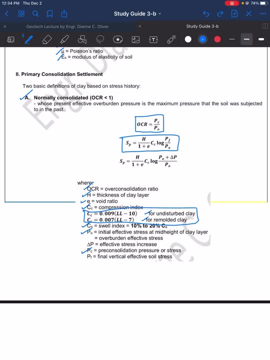 the maximum there. then we have here the uh, the p sub f. p sub f is the final vertical effective soil stress and this p sub f, this piece of f here is equal to p sub o plus delta p. so that's why here in our third formula here we have: s sub p is equal to h over one plus e c sub c. log of p sub o plus. 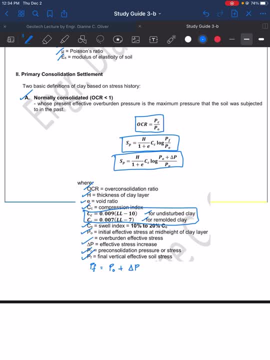 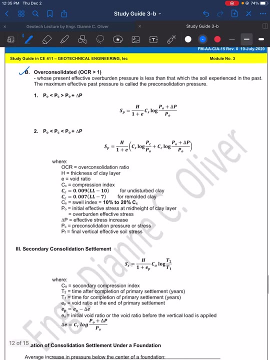 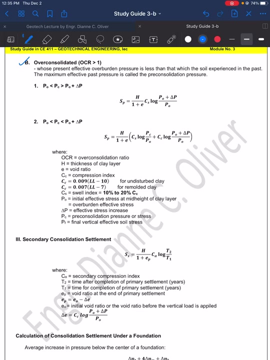 delta p over p sub o, wherein delta p is the effective stress increase. okay, so in order to fully uh memorize and understand this, we will solve sample problems later on. next, the letter b. we have the over consolidated and wherein ocr is greater than one, so over consolidated, whose present effective overburden pressure is less than. 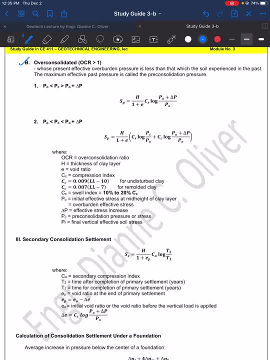 that which the soil experienced in the past years or in the past. the maximum effective past pressure is called the pre-consolidation pressure. okay, or p sub c. so we have the p sub c, pre-consolidation pressure, or stress. so we have another two cases here. the first case here is when p sub o is less than p sub c. 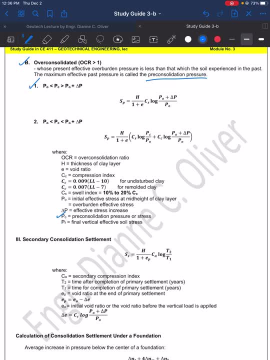 and p sub c is greater than the p final. remember this is the p final, or that is p sub o plus delta p. if that satisfies our condition, or if that condition has been satisfied, then use this formula: s sub p is equal to h over 1 plus e c sub s log of p sub o. 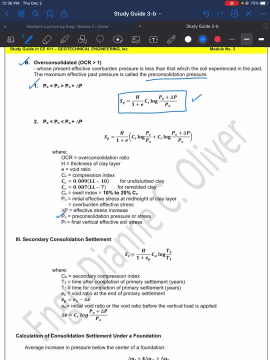 plus delta p over p sub o and again c sub s, there is swell index. okay, we have a second case. we have the p sub o, or the initial effective stress is less than the pre-consolidation pressure or stress, and that pre-consolidation pressure or 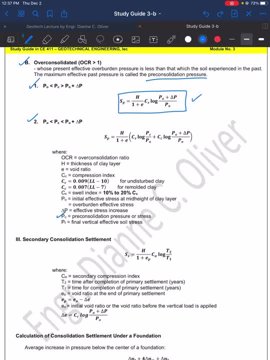 stress is less than the p final or the p sub o plus delta p. and if this case here has been satisfied, the situation there there, then this is: our formula: s of p is equal to h over 1 plus e, multiplied with c sub s log of pc over po. 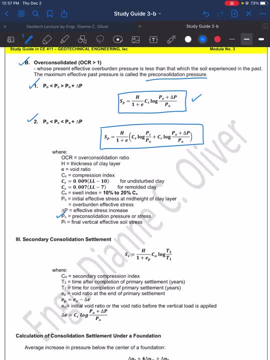 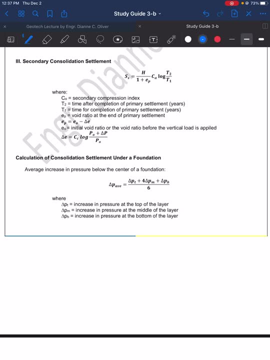 plus c sub c. log of po plus delta p over p sub o. let's go to the third one. here we have the secondary consolidation settlement. again, if you recall, this is our plastic deformation. this is the temporary one and we need time to have a permanent. i should say permanent okay. 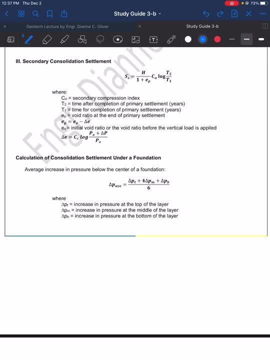 so we need time to have a permanent settlement. so that's why we have the formula here: s sub s is equal to h over 1 plus e sub p times c. sub alpha log of t sub 2 over t sub 1, wherein c alpha is the secondary compression index. 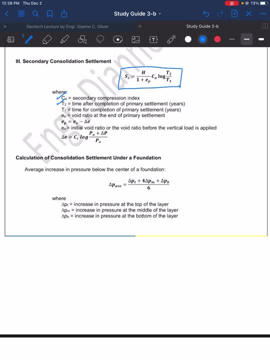 t sub 2 time after completion of primary settlement, that is in years. p sub 1 time for completion of primary settlement in years. so t sub 2 is after the completion and then t sub 1 is for the completion. e sub p is the void ratio at the end of primary settlement. 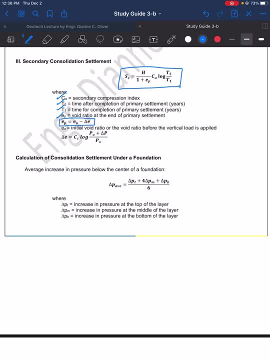 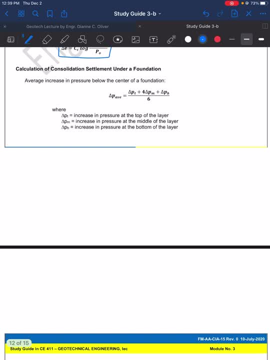 and we have the formula for delta e here as c sub c log of p sub o plus delta p over p sub o calculations of consolidation settlement under a foundation. so we can use this to approximate actually average increase in pressure below the center of a foundation. delta p average is equal to. 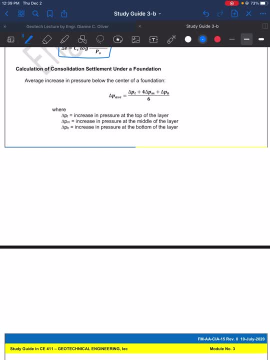 delta p sub t plus 4 delta p sub m plus 4 ani p. uh, no, no, that's plus delta p, piace di rhythms. uh, the average increase in pressure in the center of the p, wherein we have delta p sub t, is the increase in pressure at the top of the layer, and then 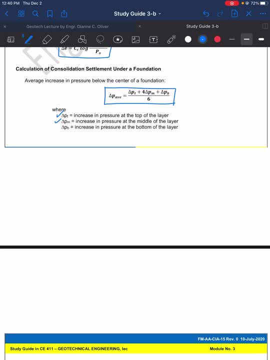 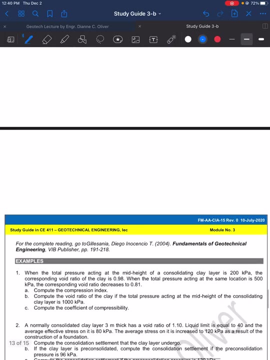 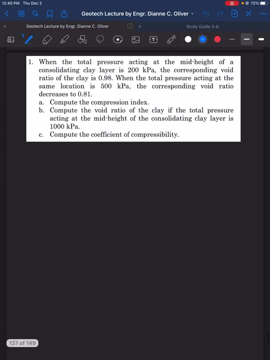 we have there the delta p sub m, that is, the increase in pressure at the middle of the layer, and then delta p sub b, increase in pressure at the bottom of the layer. okay, so that's for the formula. let's uh answer the sample problems. so i have prepared five sample problems and let's try to solve them one by one. 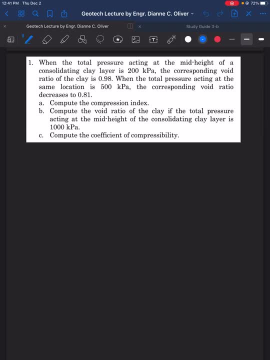 these. there are formulas that i wasn't able to mention, but uh, you can have it from our sample. problem number one: when the total pressure acting at the mid-height of a consolidating clay layer is 200 kilopascal, the corresponding void ratio of the clay is 0.98. 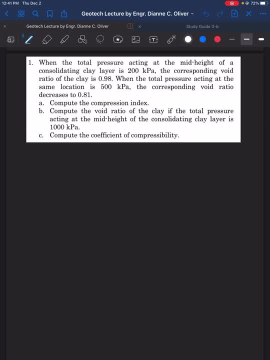 so if we write that one, the um total pressure acting at the mid-height of consolidation layer is 200 kpa. so for letter a we have pi, or maybe let's put it first: pi is 200 kilo pascal. the corresponding void ratio of the clay is 0.98. so at p1 e sub 1 is 0.98. 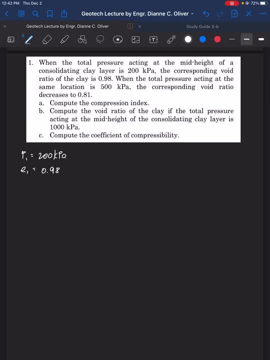 when the total pressure acting at the same location is 500 kpa, the corresponding void ratio decreases to 0.81. so that is 500, then e sub 2 is equal to 0.81, okay, okay. letter a: compute the compression index. letter b: compute the compression index. review your. 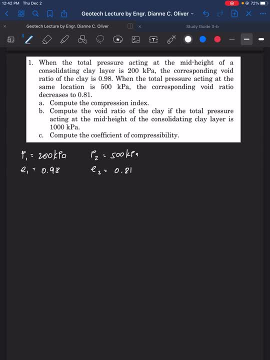 80h of k intext. lol. compute the void ratio to play if the total pressure acting at the mid height of the consolidating layer is 1000 dpa. letter c: compute the compression or compute the coefficient of compressibility. so for letter a we have there the compression index with the given p and void ratio. 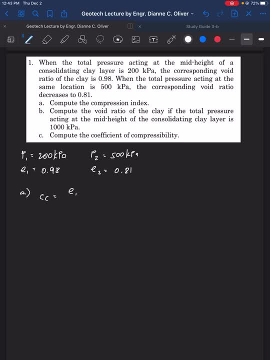 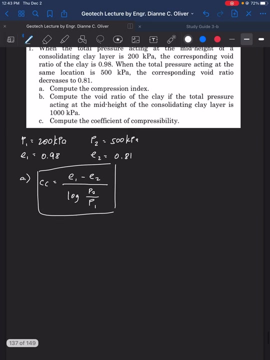 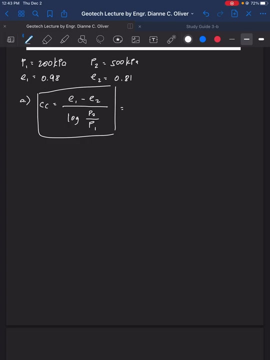 so c sub c is equal to e sub 1 minus e sub 2 will over log of p sub 2 over p sub 1. okay, so that's the formula. okay, so that we will just substitute the values. that is equal to e sub 1 is 0.98 minus 0.81. 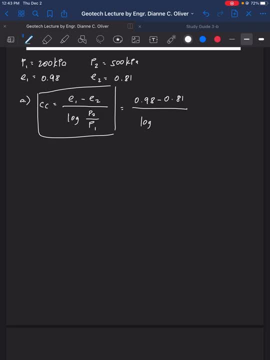 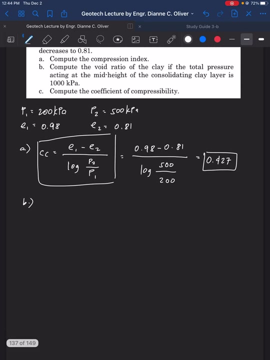 all over log of p sub o, of log of p sub 2. so that is log of 500. all over p sub 1 is 200. so to compute that we have the final answer: 0.427, and it is unitless. now let's go to letter b. letter b is compute the mid. 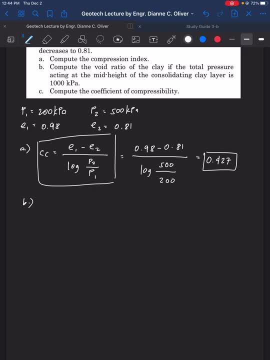 height or compute the void ratio of the clay. if the total pressure acting at the mid-height of the consolidating clay layer is 1000 kilopascal, okay, so it's looking for the void ratio acting at the mid-height of the consolidating. so let's take the answer here. 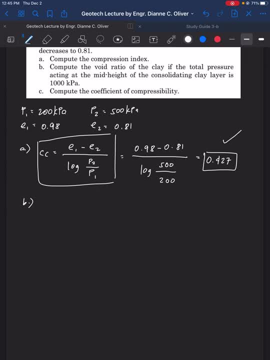 because it means that it is the, the uh cc for the difference of e sub 1 and e sub 2. so let's put here: 0.427 equals our e sub 1. there is 0.98 minus e sub 2. then we have here log of the pressure experience. 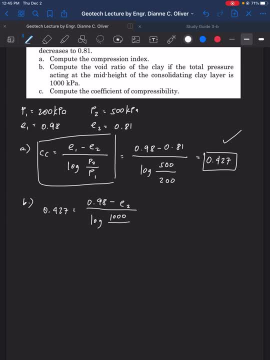 so this is 1000 over the original one. we have 200, so that is equal to. so e sub 2 is equal to 0.68. next, number three or letter c, compute the coefficient of compressibility for coefficient of compression compressibility. coefficient of compressibility for the compression coefficient. 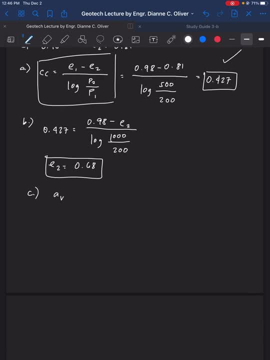 we have the formula: a sub B equals Delta, E over Delta, so our Delta is: is the difference of the two deltas, so are the two. e to void ratio is: that is point ninety eight minus zero, point eighty one, all over 500 minus. so that is equal to zero, point zero, zero, zero. 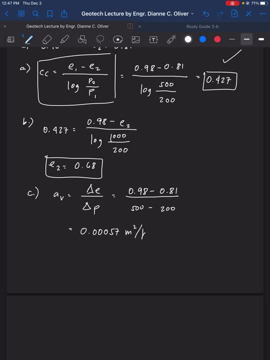 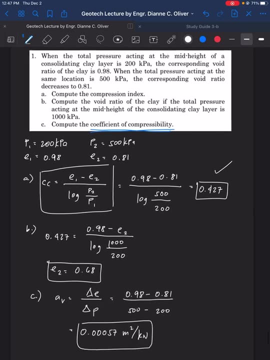 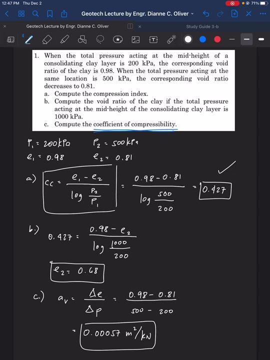 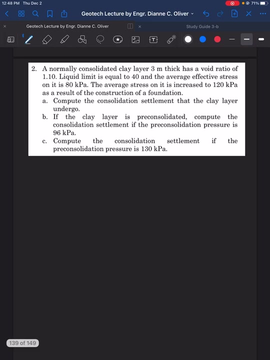 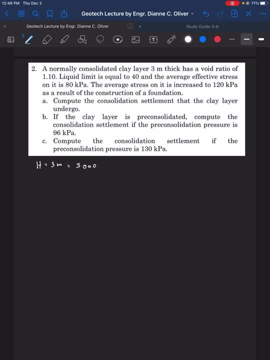 Then we have the void ratio. E is equal to 1.10.. Liquid limit is equal to 40.. Then we have the average effective stress on. it is 80 kilopascal. Average effective stress. delta or not, that is P sub O. 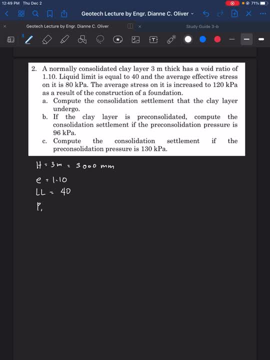 Average effective stress. so P sub O, is 80 kilopascal. Then the average stress on it is increased by 120 kPa as a result of the construction of a foundation. So that is our P final. Our P final is delta, or that is, let's start with P sub O plus delta P. 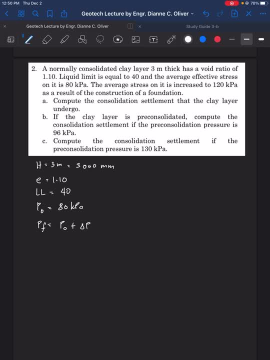 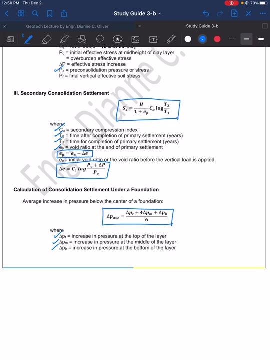 So where is So? the first question here is compute the consolidation settlement that the clay layer undergo. So we have three broad categories a while ago. We have the elastic, the secondary and the primary settlement. So which among those formulas are we going to use? 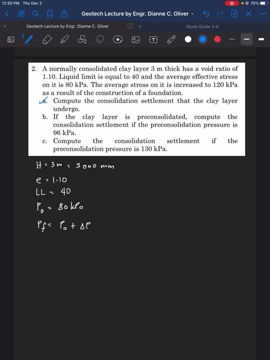 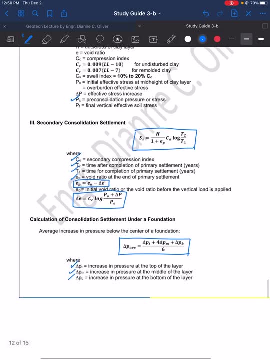 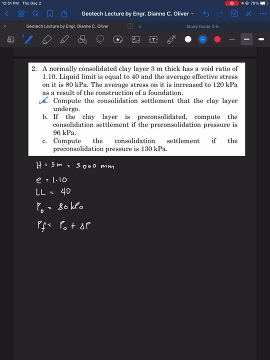 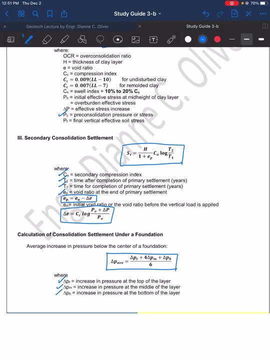 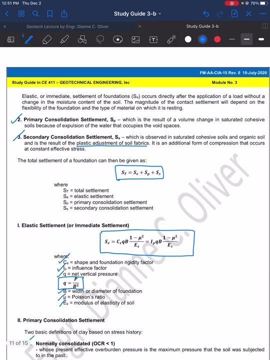 So we cannot use the secondary. because We cannot use the secondary because There's no time given in the problem, So eliminated for the secondary consolidation settlement. How about the elastic? You can also eliminate that because of no presence of stress. So we need to calculate it by using this wasson's ratio. 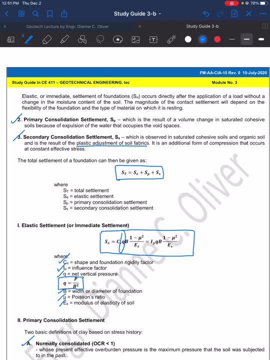 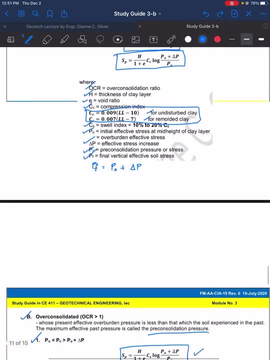 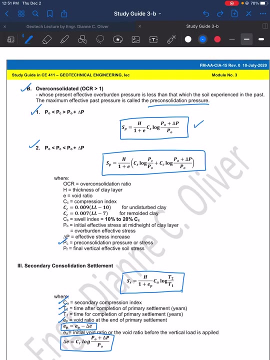 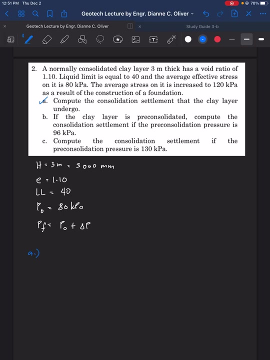 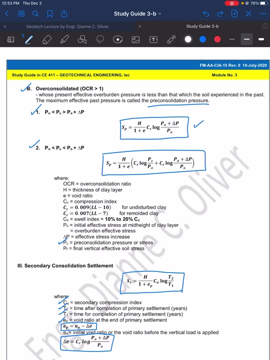 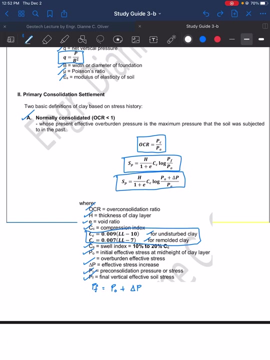 That is the small cube here and the was-sons ratio. Therefore, we can conclude that we are going to use the normally consolidated. So we will be using the primary consolidation settlement. So we will be using the primary consolidation settlement, So SP. And the formula for SP is: let's take the formula We have the H over 1 plus. 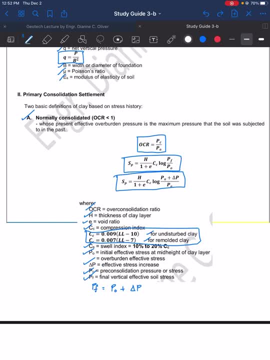 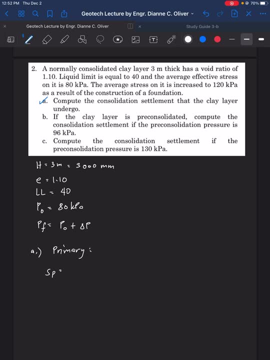 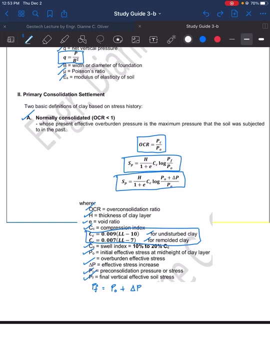 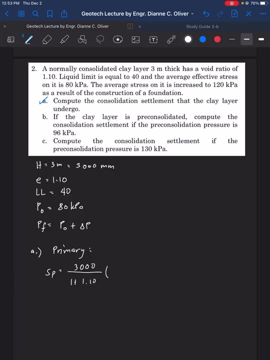 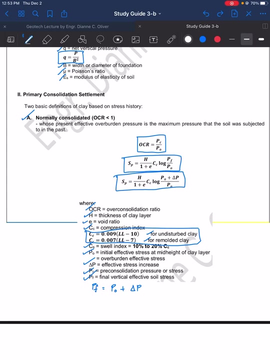 E 100.. So SP is, we have the H. well, it's 3,000 mm all over 1 plus 1.10.. And it's our CC, CC or CS. Okay, so we have here the CS of 0.20% of CC. 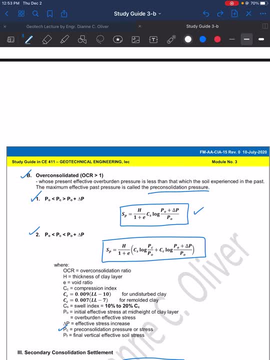 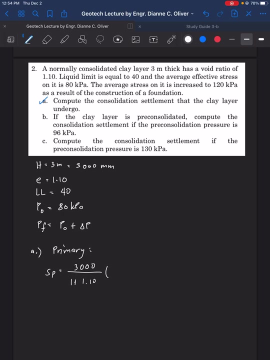 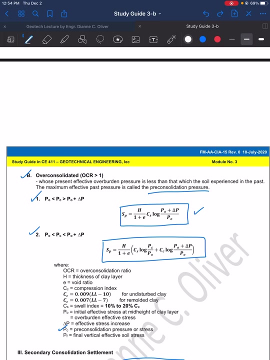 So our P sub O, how is our P sub O delta P and Okay, Okay, So, given P O, we have our delta P plus P sub O. what else PC? So we cannot compare it here. 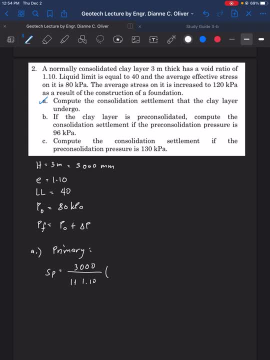 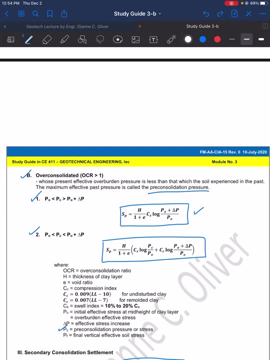 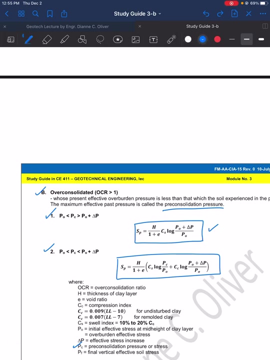 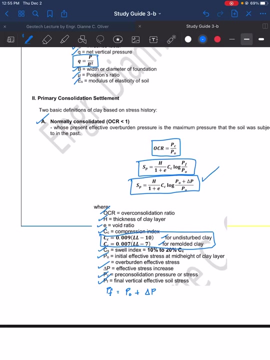 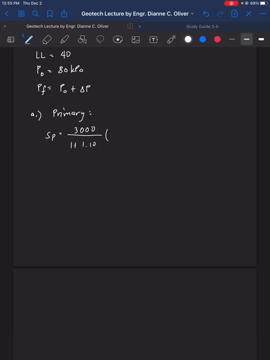 So there is no mention of preconsolidation. Therefore, we are going to use: since there is no mention for P sub C, we can then conclude That this is the one being used. So SP 3,000, or I should write the formula first. 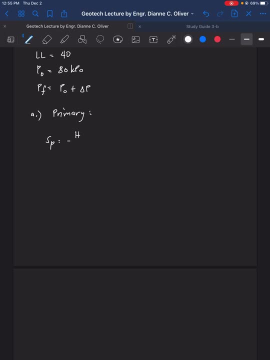 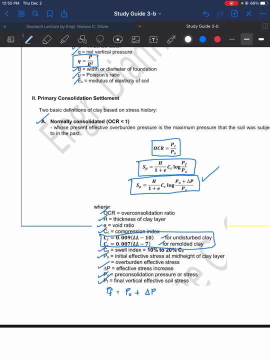 So S sub P is H over 1 plus E CC log. So CC log of PF over P sub 0.. Let's see if we did it right. Okay, so we did it right. Now, what else is? we need to have the value of C sub C. 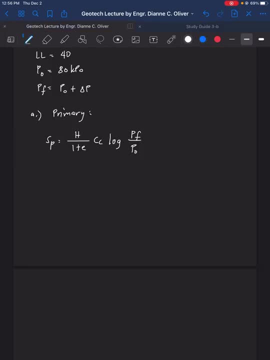 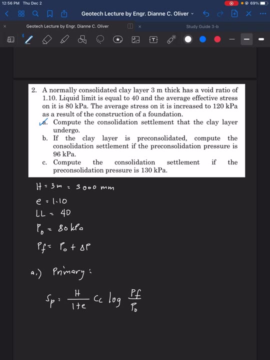 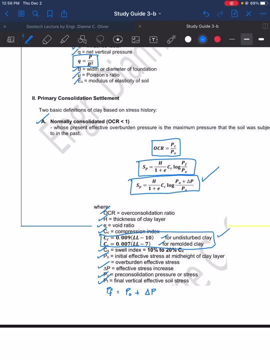 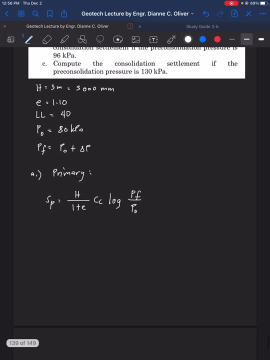 And from this problem. the soil here is an undisturbed soil layer. Okay, So if it is an undisturbed play, therefore it is point zero, zero, point zero, zero nine times l, l minus ten. so if it is undisturbed play, then we can now compute for c sub c, so c sub c equal to 0.009. 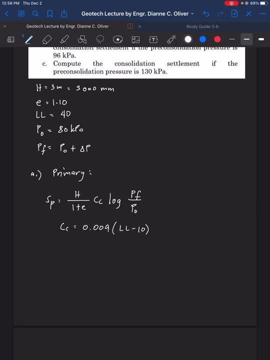 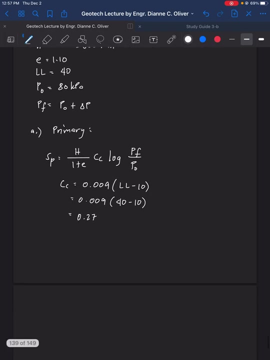 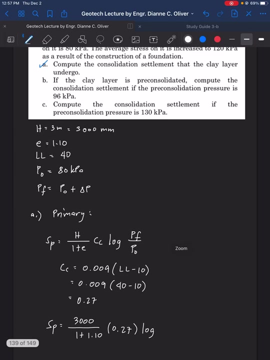 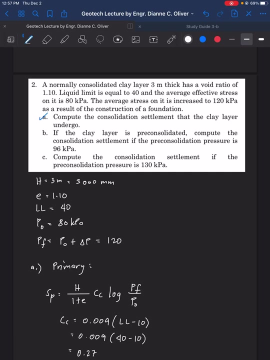 l, l minus 10.. so 0.009 liquid limit given 40 minus 10, that is equal to: 40 minus 10 is 0.27. so we now have sp. a sub p is equal to 3000. all over 1 plus 1.10, 0.27 log of delta. so p delta here, so it becomes 120 dpa. 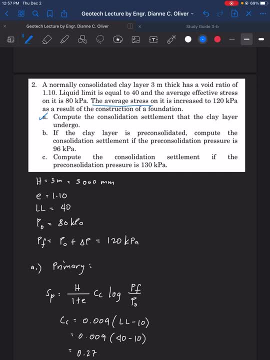 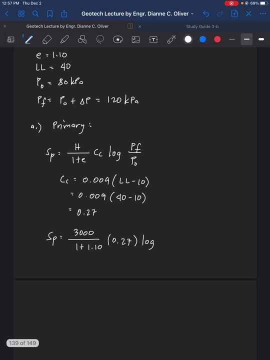 so it's one. the average stress on it is increased to 120 epa, so that becomes p, final p sub o plus delta. so log of 120 all over p sub o 80. so s sub p equal to 3000, so 3000 over 2.1. 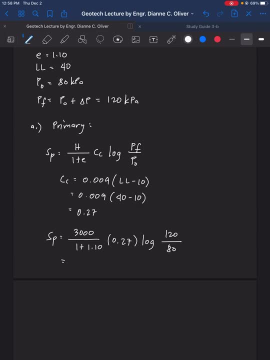 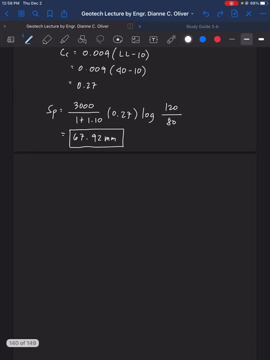 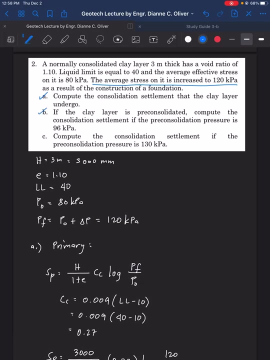 times 0.27, log of 120 over 80.. so that is equal to 67.92 millimeter. millimeters. because we have here the three meters becomes 3000 millimeters. okay, let's go to letter b for letter b, if the clay layer is pre-consolidated, 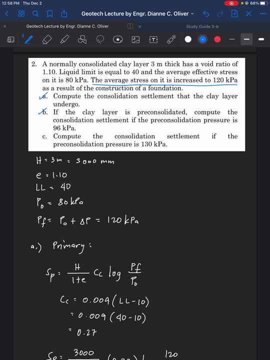 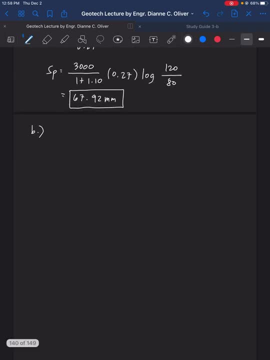 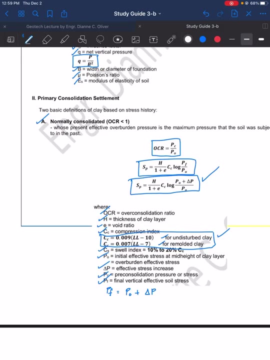 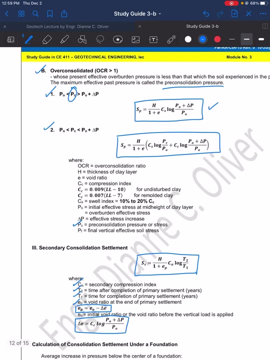 compute the consolidation settlement. if the pre-consolidation pressure is 96 kilopascal, so this time pc is given, so pc is 96 kilo pascal. and if pc is given we won't use our the normally consolidated clay. we will have the over consolidated. so we will check which among 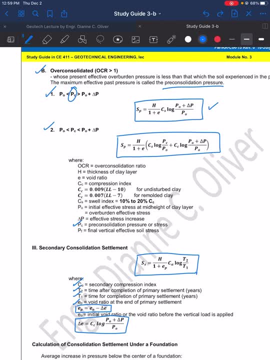 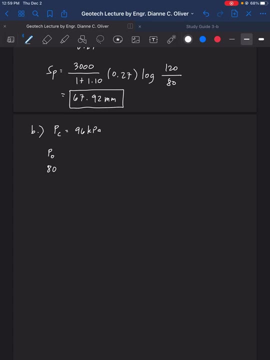 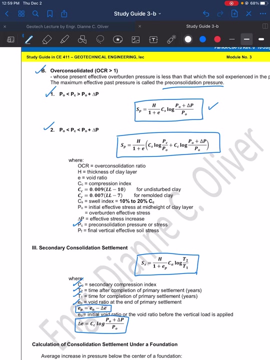 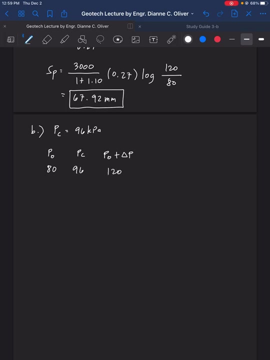 these two cases feeds. our P sub oh is a P, so P sub oh it's a P. our PC is 96. and what else together? P sub Oh plus delta P, so P sub Oh plus delta P, that is 120. so this is which one P sub C is greater than P O, but less than P O plus. 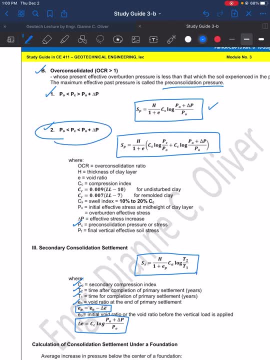 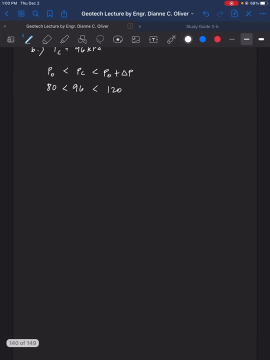 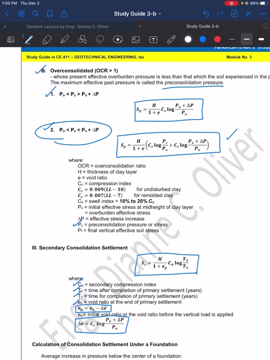 Delta P. so this is the case. the second one, therefore, we're going to use this formula, so s sub P, so s sub P is equal to the formula H over 1 plus E, and then multiply it with CS log, PC over P, O plus we have CC log of P. final. 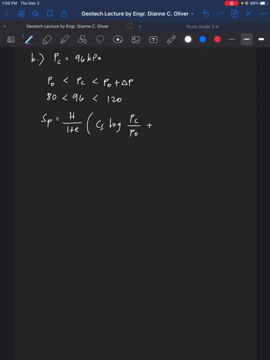 over P sub O. this P final here is P sub O plus Delta. ok, so this is 3001 plus one point. then times CS of. then what is CS? let's take the maximum, so let's put CS here. maximum, that is point. that is 10% to 20%. so this is 20%. 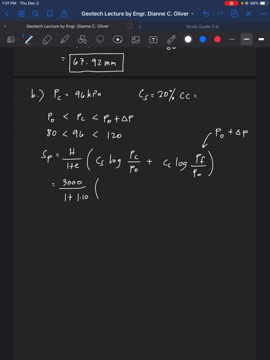 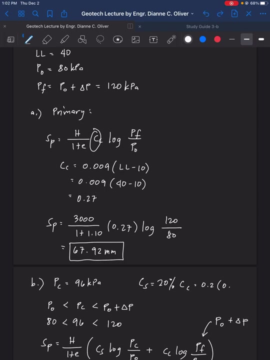 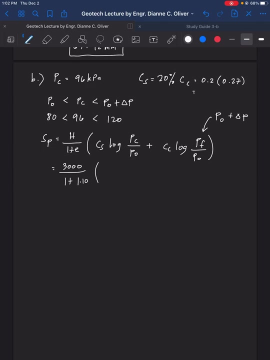 of CC is equal to. so what is 0.2 of C, sub C of 0.27, 57? that is CC 0.27. so 0.2 times 0.27 is 0.054. so CS here is 0.054. 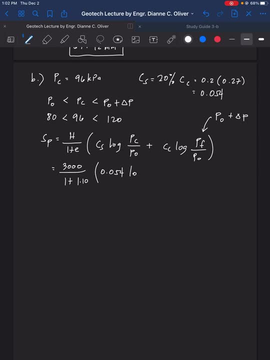 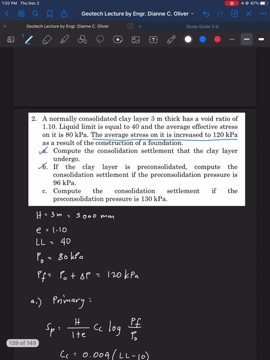 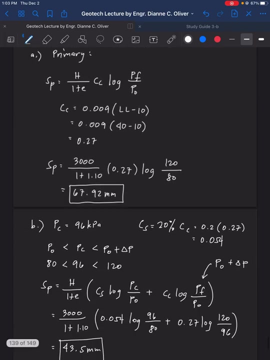 log of 96 over 80, plus CC, CC of point 27, look of 120 over 96, so that's equal to 43.5 millimeters. is that's for letter B? next letter C. letter C: here is complete the consolidation settlement if the pre consolidation pressure is 130, so PC is.